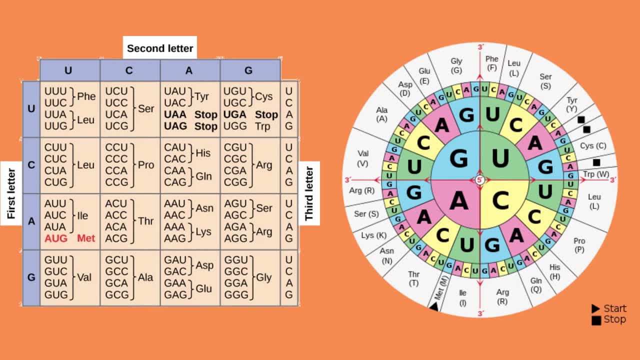 using a codon table or a codon wheel. We will use the same strand of mRNA in both cases for simplicity, to make sure you understand the idea behind both of these. Before we do anything else, we need to find a starting point. We need to find a starting point for the mRNA. We need to find a starting point. 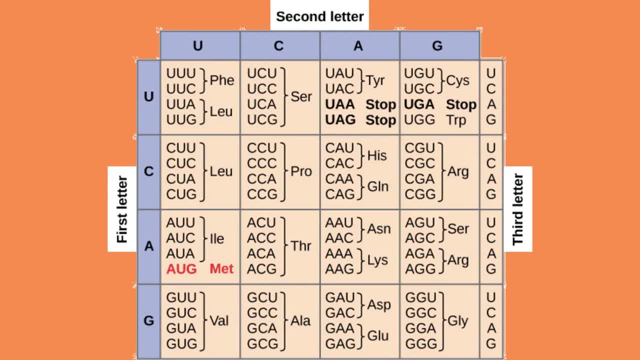 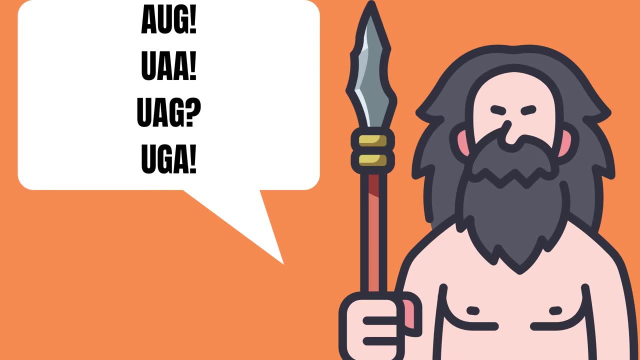 codon and a stop codon. From the table we can quickly notice that the start codon is AUG. The stop codon will either be UAA, UAG or UGA. For some reason, thinking about a caveman helps me remember all four of these start and stop codons. The space in between the start and stop codon is known as a. 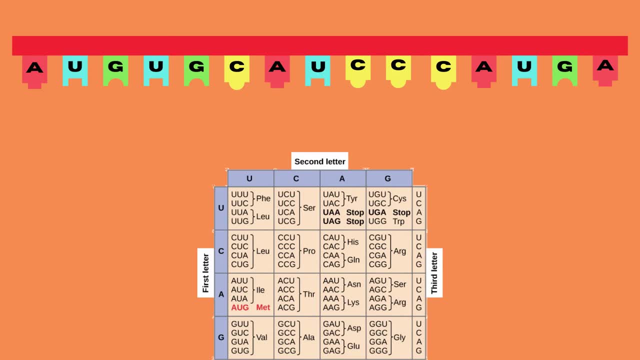 reading frame. So, starting with the codon table, we simply read it from the left to the right. The start codon codes for methionine. the second triplet is UGC. By looking at the table here, here and here, we can see that the second amino acid is cysteine. Then comes AUC. 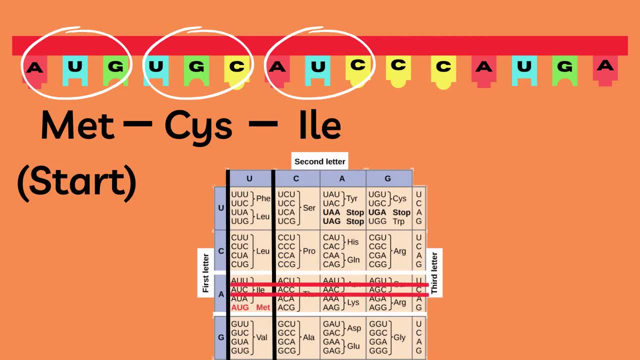 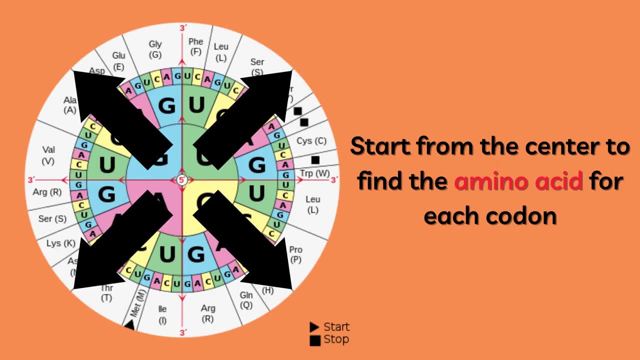 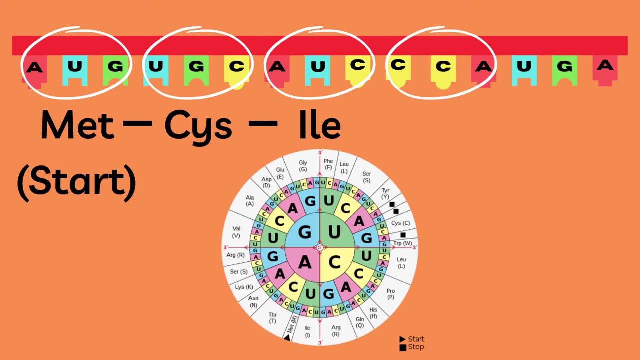 Now we look here, here and here to see that the next amino acid is isoleucine. The codon wheel is almost even more intuitive. You simply read from the center outwards. Let's use the same example to read out the final two codons. So next comes CCa, By simply. 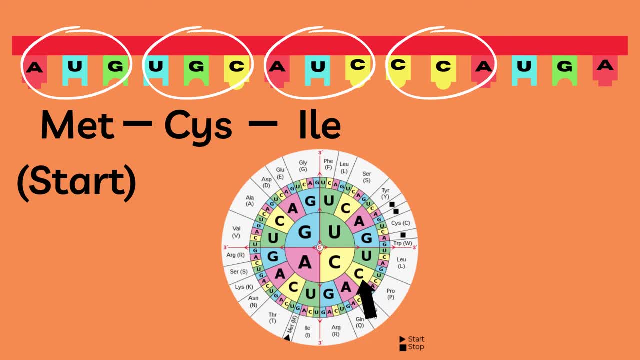 starting from C, going to the next C and all the way out to A, we see that the next amino acid in the chain is proline. The final codon is UGA, which you might remember, since it sounds rather Kemal-like UGA. Anyway, let's read it out, just to ensure that we know how to use the wheel as well. 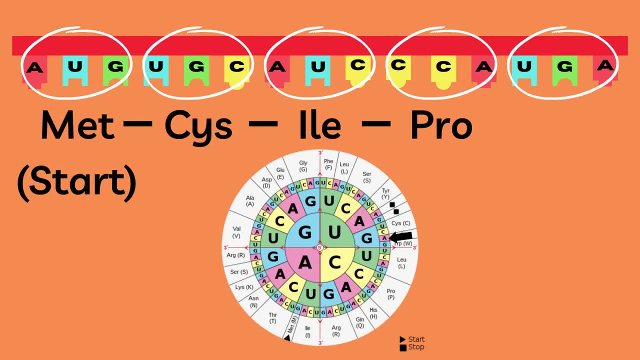 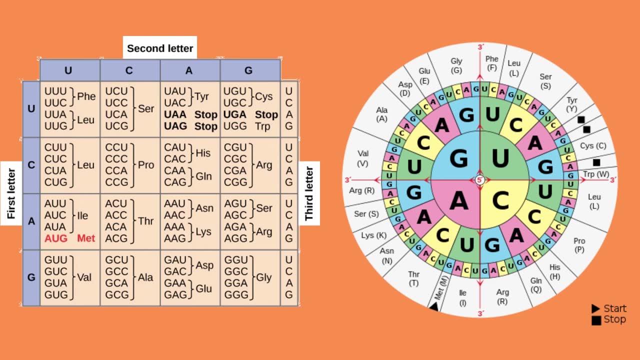 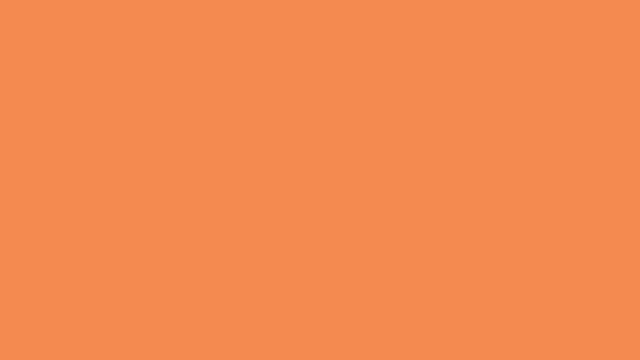 So we simply read U to G to A and find this little square which, if we look here, we can see, means stop. Congratulations, You now know how to use a codon table as well as a codon wheel. If you want to learn more about how this process is actually carried out inside of the ribosome, check out this video Until next time.